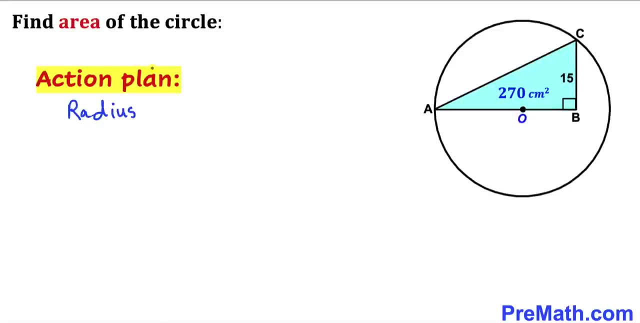 And here's our action plan. Before we calculate the area of this circle, we must find the radius of this circle, And here's our very first step. Let's focus on this blue triangle ABC. we know it's this side. length b. c is 15. now we are going to calculate this side length a, b and. 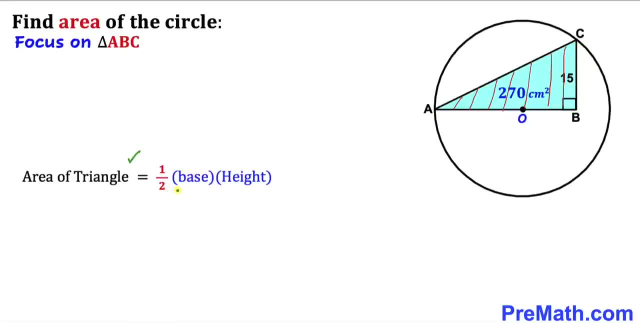 now let's recall the area of a triangle formula: area equals to a half times a base times a height, and in our case our area is 270, our height h is 15, and now we are going to find out our base b. so let's go ahead and fill in the blanks in this formula. our area is 270, equals to a half. 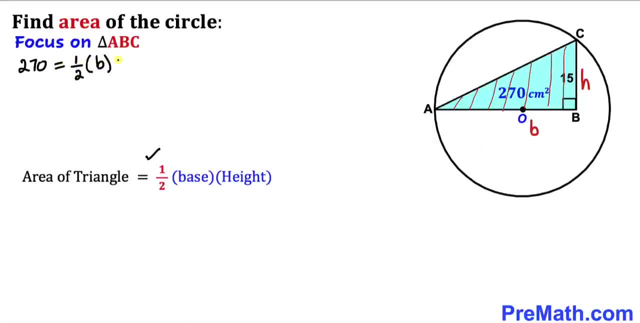 times our base is b times our height. h is 15, so therefore we can write this thing as 270 equal to 15 divided by 2 times b. now let's go ahead and multiply by the reciprocal formula of 15 divided by 2, which is same as 2 divided by 15, and I'm going to multiply on this side. 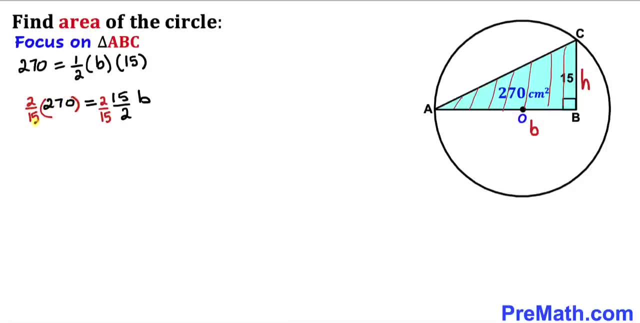 2 divided by 15 as well, and here these cancel out. so therefore, our b value turns out to be: if we simplify the left hand side, that is going to give us 36 centimeter. so thus our this a b length turns out to be 36 centimeter. and here's our next step. I have extended this line. 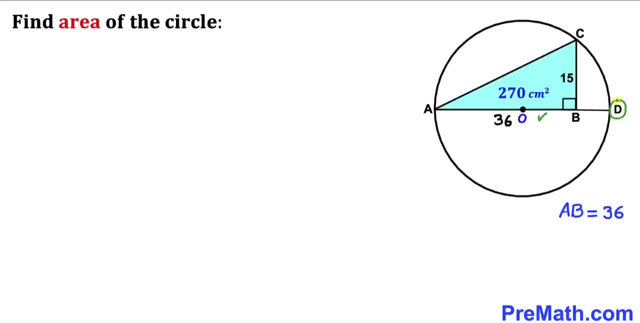 a b all the way to this point d and as a result, we got this a- d as the diameter of this circle, with the center out. and in this next step I have connected this point c with this point d. this recalls the Thales theorem. according to this theorem, if a, b and d are three distinct, 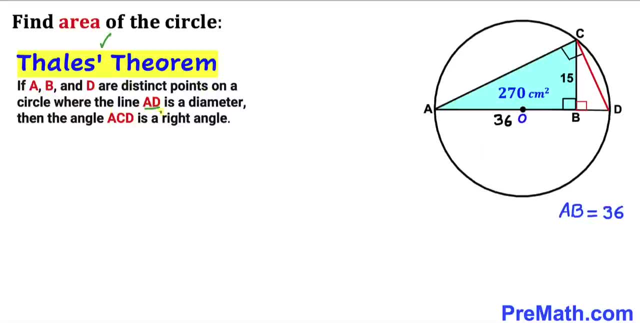 points on a circle where the line a, d is the diameter, then the angle a, c, d is a right angle. as you can see in this given diagram, a, c and d are our distinct point on the very same circle and a- d is our diameter, so no wonder our this angle. 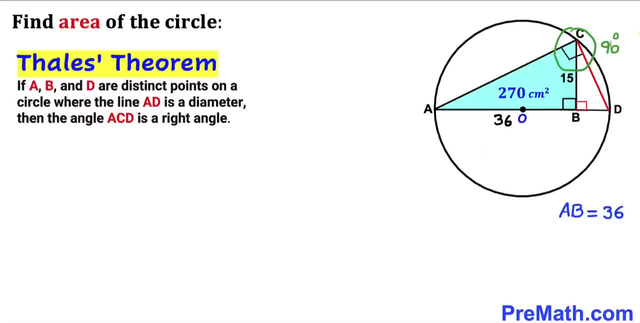 c, d is going to be 90 degree angle. and now, in this next step, let's assume that alpha and beta are our two complementary angles. in other words, some of these angles, alpha plus beta, must be equal to 90 degrees. now let's assume that this angle in this blue triangle is alpha. we know this is. 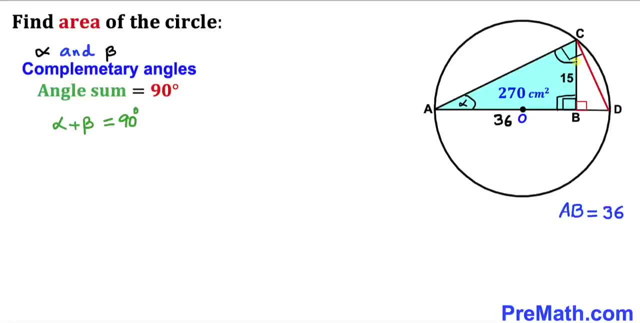 our 90 degree angle. so therefore, this angle is going to be our angle beta. and now we can see that this whole angle is 90 degrees. this angle is a beta, so therefore this angle has got to be our angle alpha. and finally, in this triangle d, b, c, this 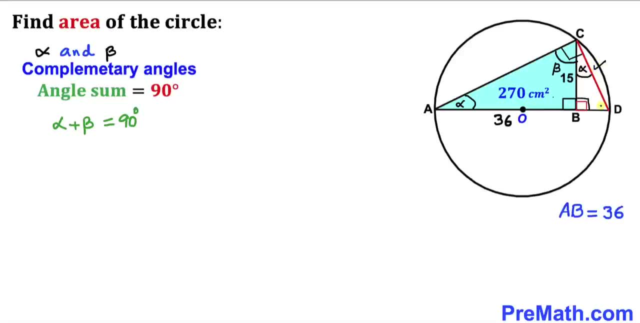 angle is 90 degrees. this angle is alpha, so therefore this angle has got to be our angle beta. and now we can see that this triangle b d is similar to this blue triangle a, b, c according to angle angle similarity theorem. and here's our next step. let's assume that this line, segment b d, is x centimeter, and since these 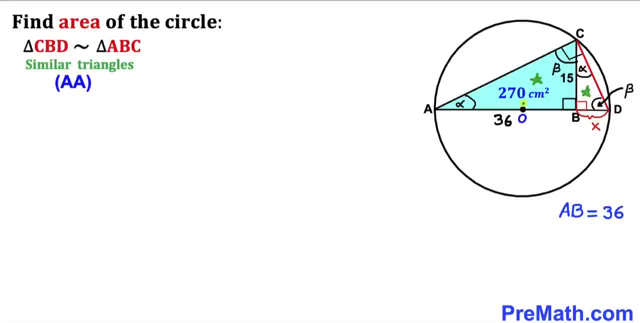 two triangles are similar, so therefore we are going to have a proportion. so therefore we're going to have a ratio of this side length, x and 15, equal to the ratio of this 15 and 36. so therefore, let me go ahead, write down: x divided by 15 equals to the ratio of 15 divided by 36. and now we can. 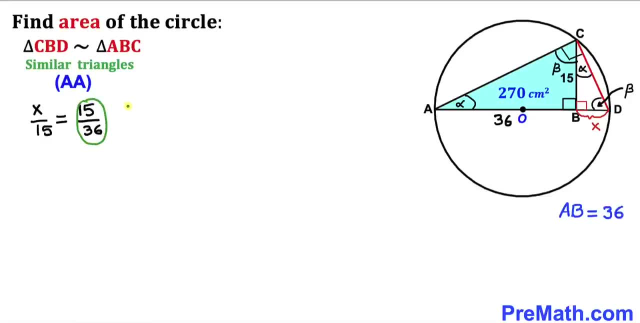 see that 15 divided by 36 could be reduced to 5 divided by 12. so therefore we can write: x divided by 15 equals to 5 divided by 12. now let's go ahead and multiply both sides by 15 to isolate x, and now we can see that this 15 and 15 is gone. so therefore our x value turns out to be: 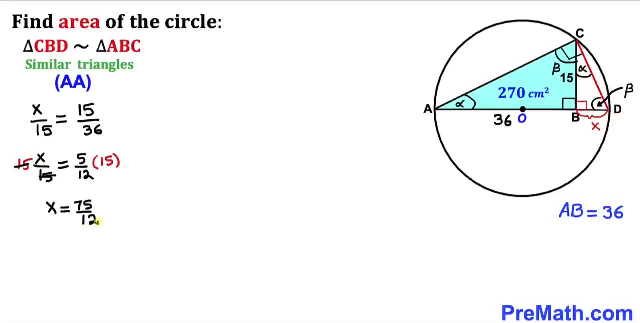 75 divided by 12 centimeter. so therefore, our this x value turns out to be 75 divided by 12. and now, in this next step, let's make an observation. we can see that this diameter ad is going to be equal to this side length ab, which is 36 plus this side length x. so therefore, our diameter ad is going: 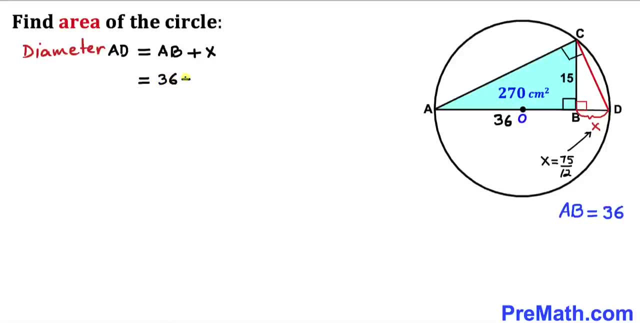 to be equal to. let me go ahead, andglio, and we can see that the diameter ad is going to be equal to. and Corinne, we know that this diameter is going to be equal to this side length x. so, therefore, our go ahead and fill in the blanks: 36 plus 75 divided by 12. and now, in this next step, I have 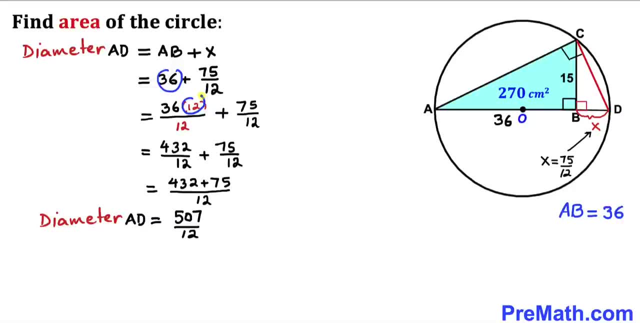 multiplied this 36 by 12 and divided by 12 as well, to get this common denominator 12. so as a result, we got 432 divided by 12 plus 75 divided by 12, and if we add these numbers on the top, we got 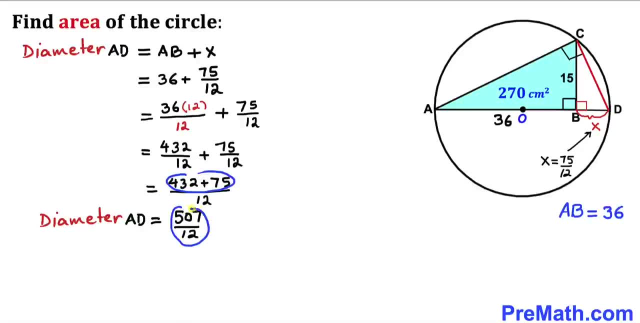 507 divided by 12. so therefore our diameter AD turns out to be 507 divided by 12. so therefore the radius R, lowercase r, of this circle is going to be half of this diameter. so we are going to divide this fraction by 2, so therefore our radius of lowercase r is going to be half of this. 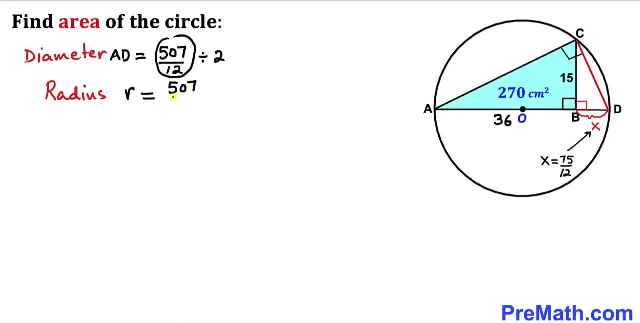 diameter. so this is going to become 507 divided by 24 centimeter. and here's our final step. let's go ahead and calculate the area of this circle. and now let's recall the area of a circle. formula: area equals 2 pi R square, where R, in our case the radius, is 507 divided by 24. so therefore the area